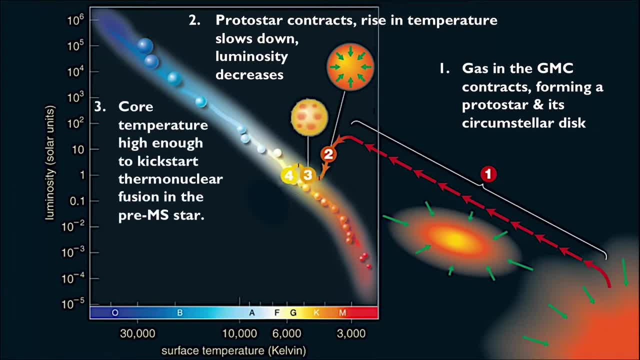 of hydrogen into helium, at which point this pre-main sequence star is finally considered a star And it lands on the zero-age main sequence line, or the Zams line. This line, usually at the leftmost edge of the main sequence, represents the point of a star's evolution at which the dominant energy 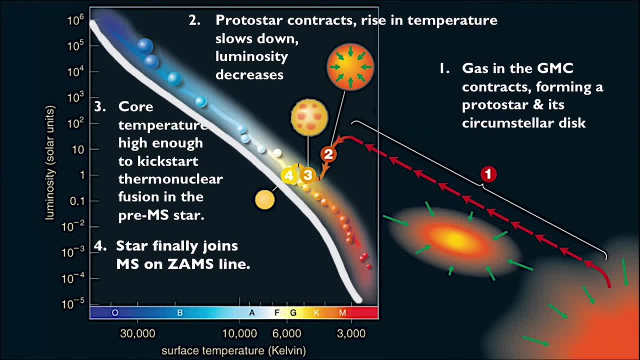 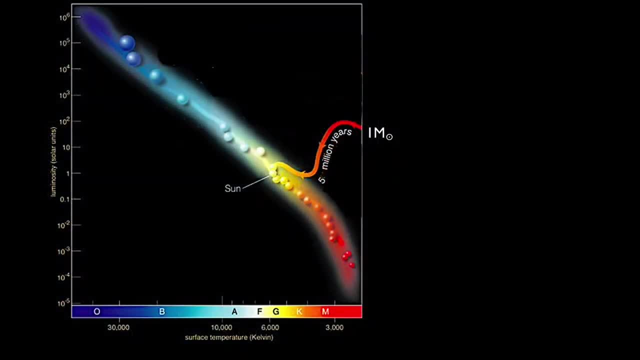 production has become thermonuclear fusion rather than the gravitational contraction that used to fuel its luminosity before. The exact path that a star follows in its pre-main sequence evolution depends solely on its mass. All the different mechanisms that determine the shape of these paths have different timescales. 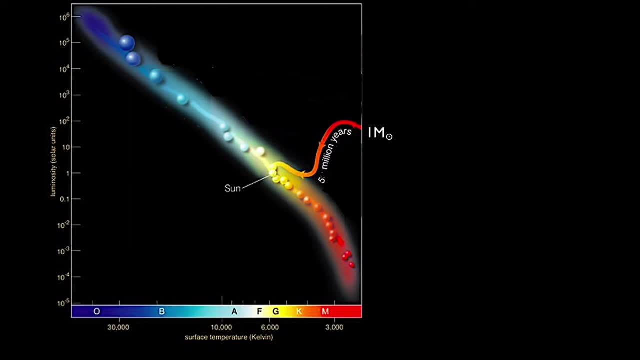 depending on the mass of the protostar that's evolving into a pre-main sequence star and then into a main sequence star. Stars like our Sun have a pretty steep evolutionary path, taking about 5 million years to evolve from protostar to pre-main sequence star to star. 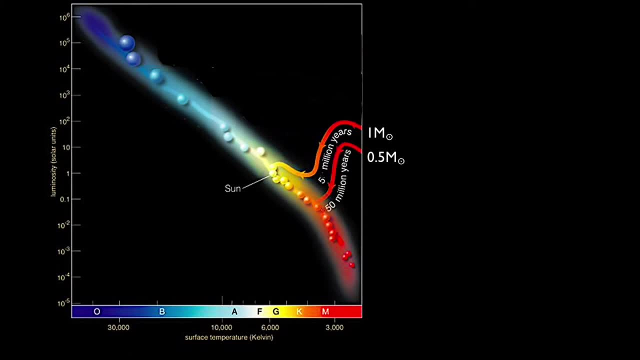 Stars that are smaller than the Sun- say of mass one-half of our own Sun- have a pre-main sequence that's more vertical than the evolutionary path of the Sun. These smaller stars would take much longer to undergo the process. Larger stars, however, tend to have a slightly less vertical. 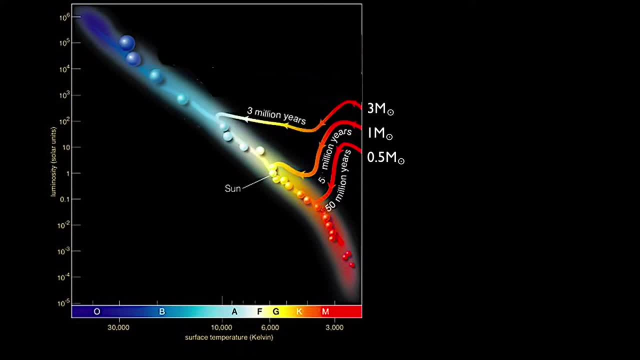 approach to the main sequence, A three-solar mass star drops in luminosity while continuing to heat up, but not as much as the Sun, And similar patterns can be seen for stars of 9 or 15 solar masses. Notice also that the bigger the star, the shorter the amount of time that it takes for it to 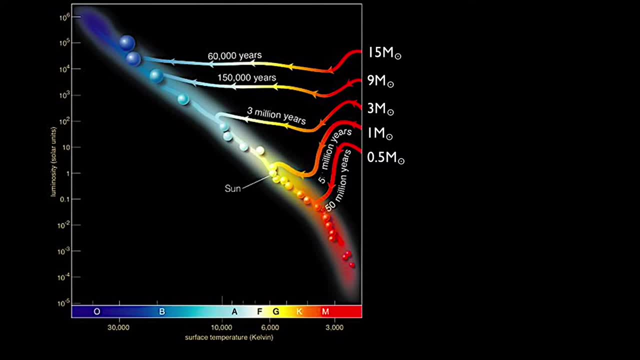 become a main sequence star Because, remember, very massive stars burn fast, burn bright and die young And for the same reason they form pretty quickly too. When we look at the pre-main sequence evolutionary tracks of all five of these differently massed 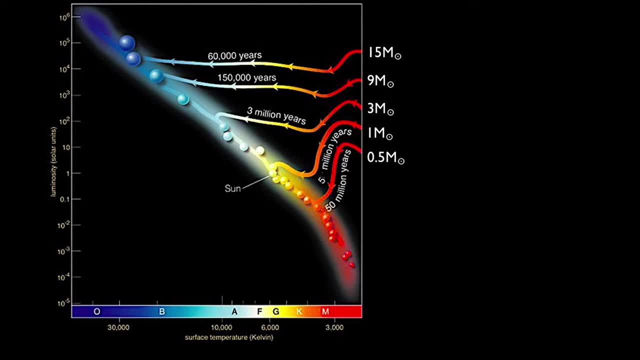 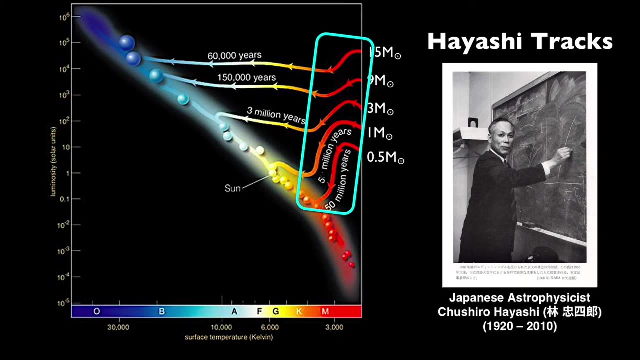 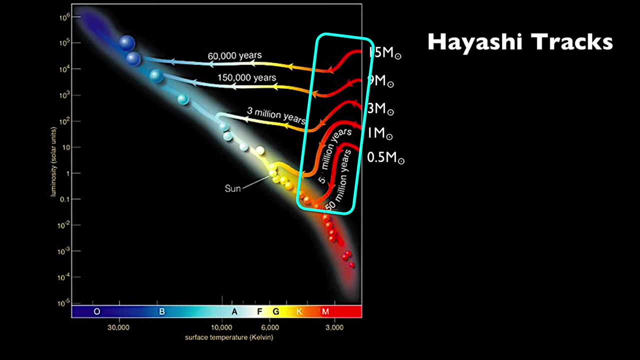 stars. there seems to be some sort of a trend where the luminosity drops a little bit as the stars continue to slowly heat up. This portion of the pre-main sequence evolutionary path is called the Hayashi track, Named after Japanese astrophysicist Chishiro Hayashi. The other trend worth noting is the 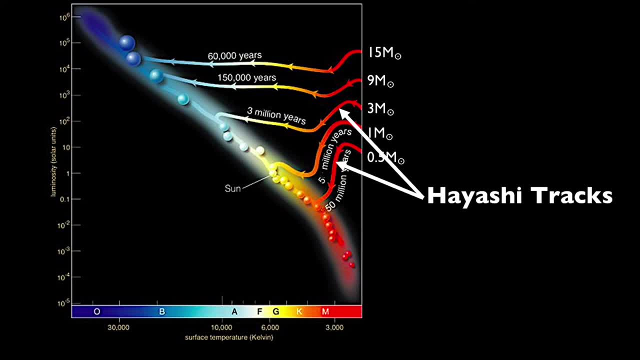 tendency of the larger mass stars to practically continue heating up at a steady rate as they approach the main sequence. This horizontal portion of the pre-main sequence evolutionary path is called the Henyei track, Named after Hungarian-American astronomer Louis Henyei.